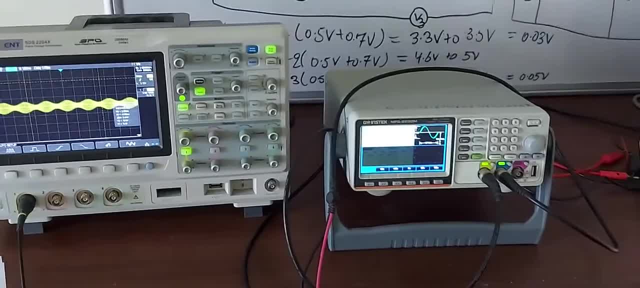 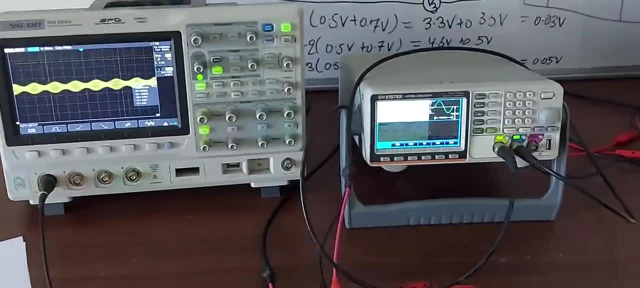 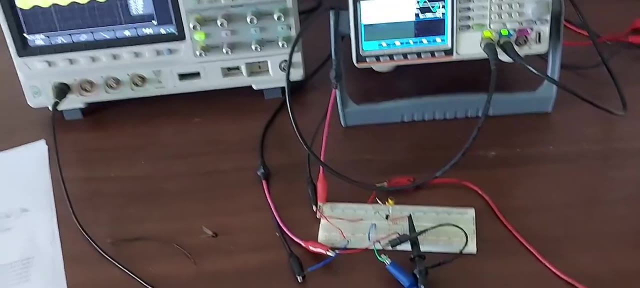 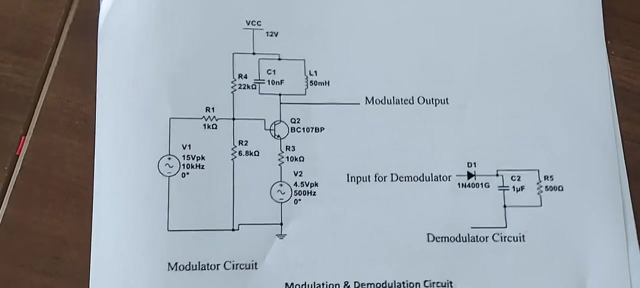 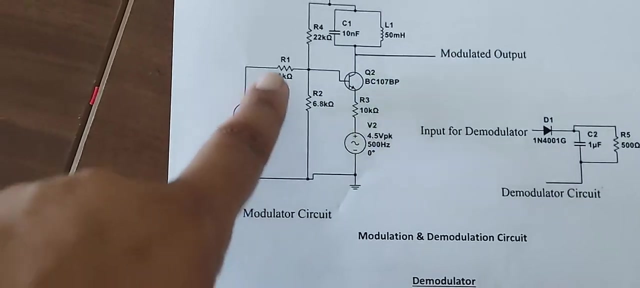 Hello guys, so this is the first lab of analog communication. This is just the demonstration of AM modulation experiment. So I will show you today how we modulate AM signal in hardware implementation. So first of all we will go to the circuit. So this is the circuit of AM modulation. As you can see, this is our transistor BC107BP and there are several resistances of different, different values. We have one capacitor and one inductor. 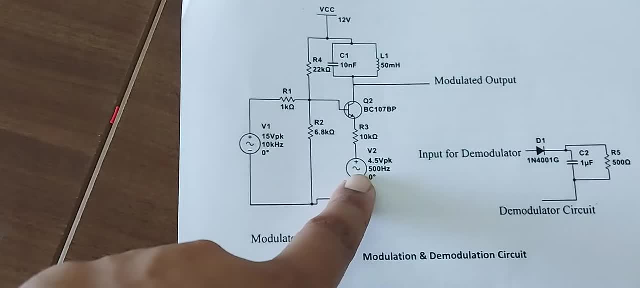 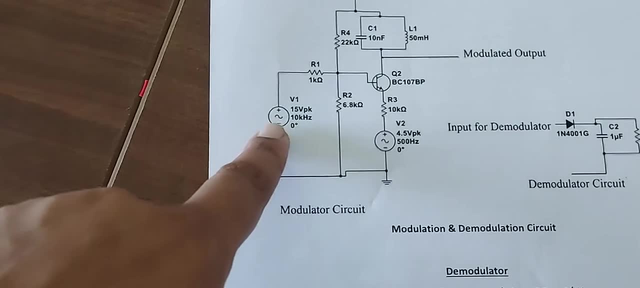 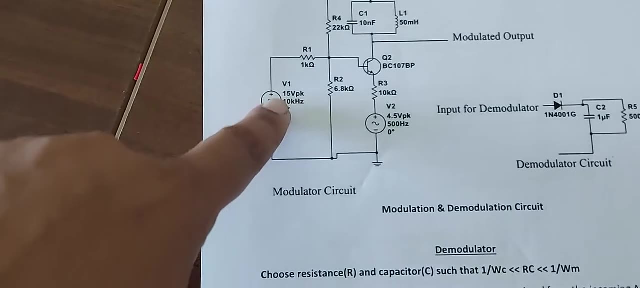 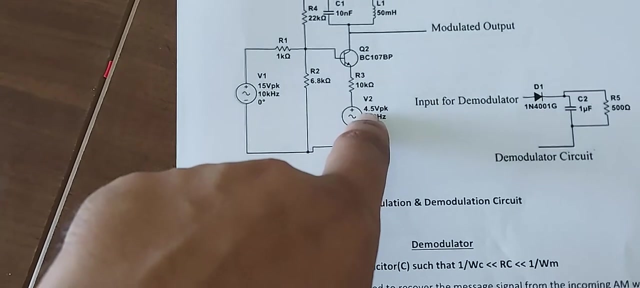 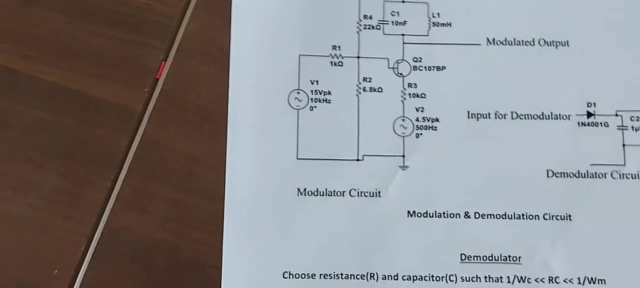 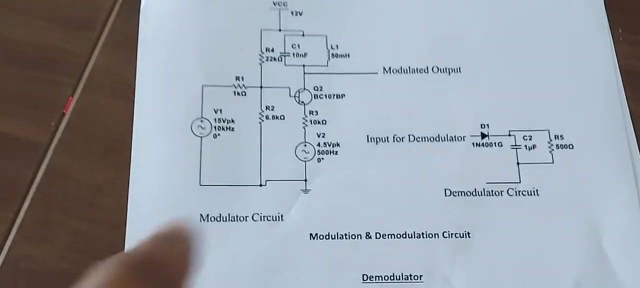 Two input. one is this: this is for the message signal- FM and AM- frequency and amplitude. This is for the carrier signal: FM and AM. As you can see- this is sorry- AC is 15 volt and FC is 10 kilohertz. right now, This by default, we kept it as 10 kilohertz. This of message signal. the amplitude is 4.5 volt and the message signal frequency is 500 hertz. Okay, and these are different, different resistors and capacitors. 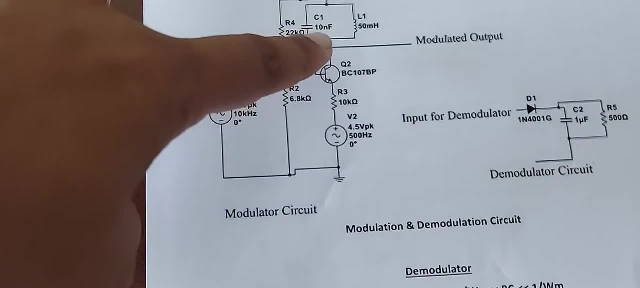 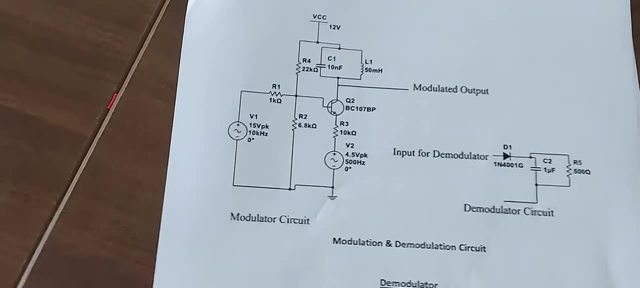 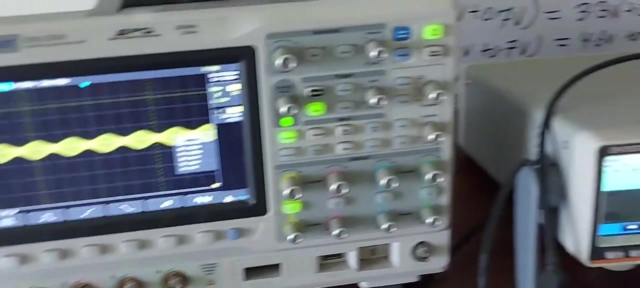 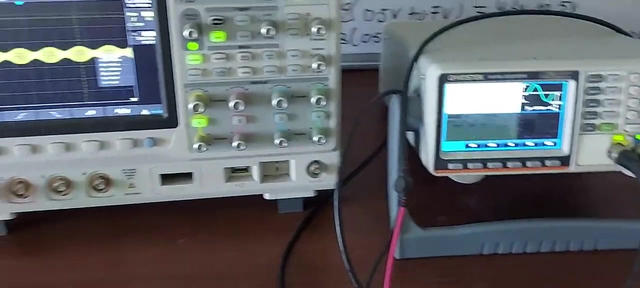 We will take output from the collector of NPN transistor. From collector of NPN transistor we will take one output. We will observe the output on CRO. So I have already shown in your last semester that we have several other other devices from where we use to generate our signal and use to observe that. So first of all I will start with this power supply. 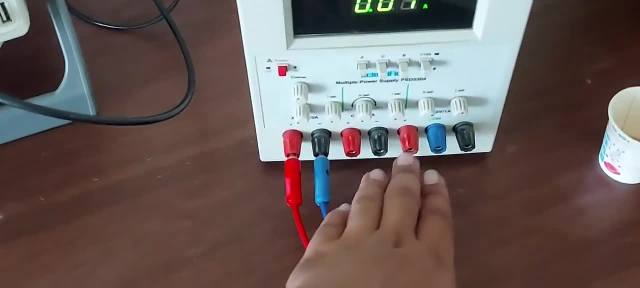 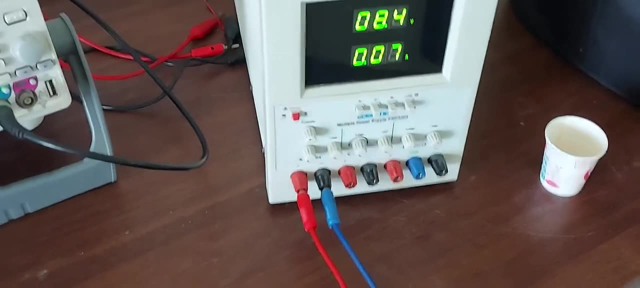 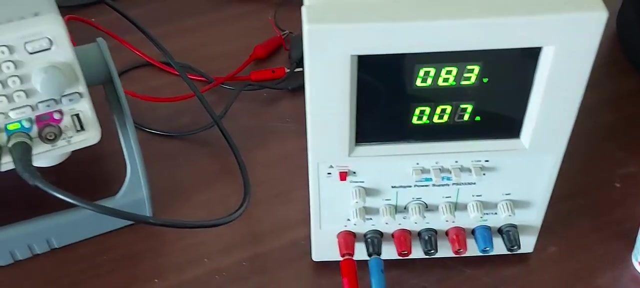 As you can see, it has three channels: one, two and three. we can take simultaneously 3 outputs from here. Right now I have connected in first channel and the output I'm giving to the circuit is 8.3 volt. We can vary this also using these things. Okay, we can vary this. 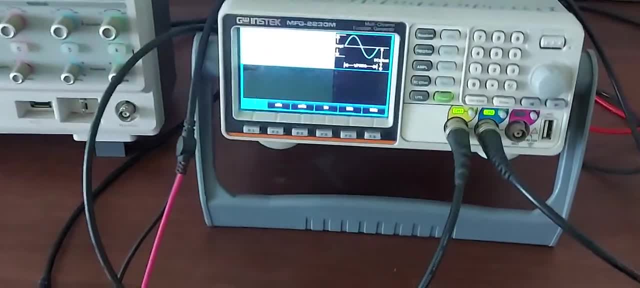 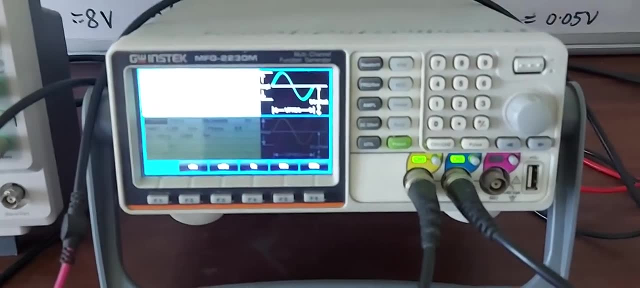 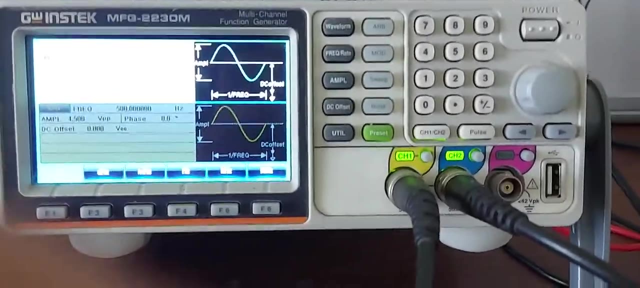 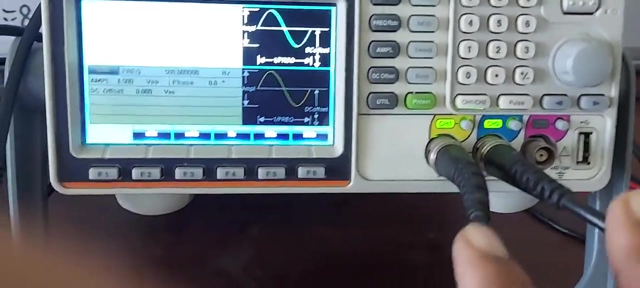 So this is one. This is second thing, is this two channel function generator? this is our function generator. okay, as you can see, we can give different frequencies and we can change the frequency and amplitude. you can see, this is the channel one, this is the channel two. I am using the channel. I am using this channel one. it is going to connect. 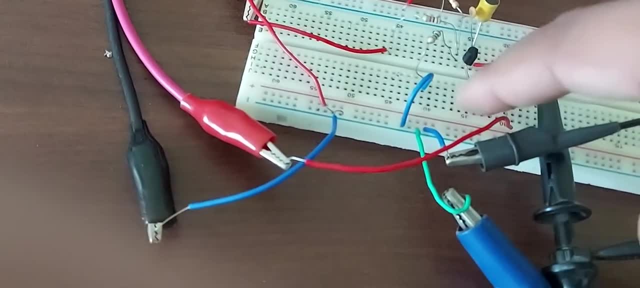 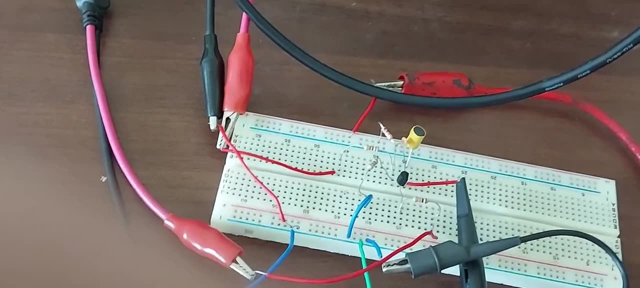 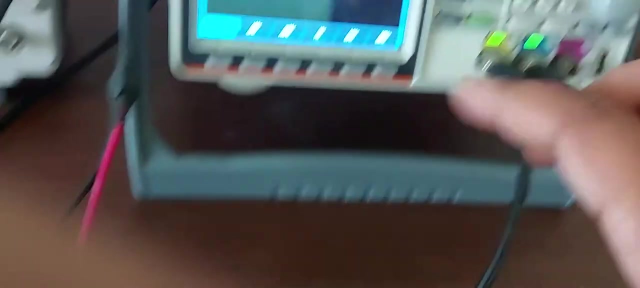 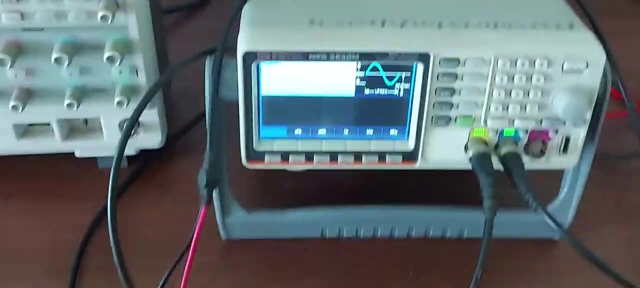 it in our circuit, as here here. so this is for message signal channel one. it will supply the sine wave and this is for the. this is connected. this channel two is connected. this channel two is connected at this place. okay, so this is for the carrier signal. okay, so, as we know, in EM modulation, message signal 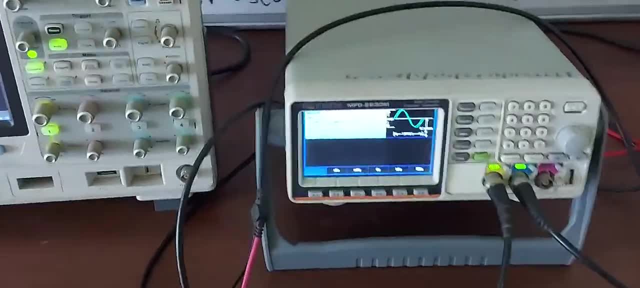 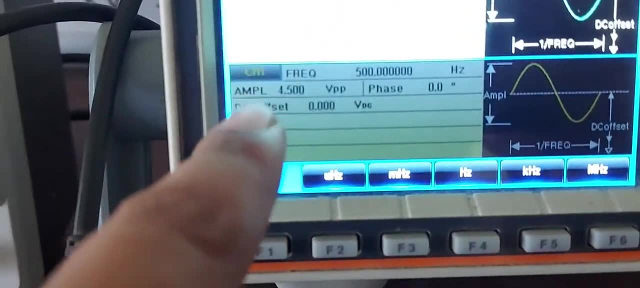 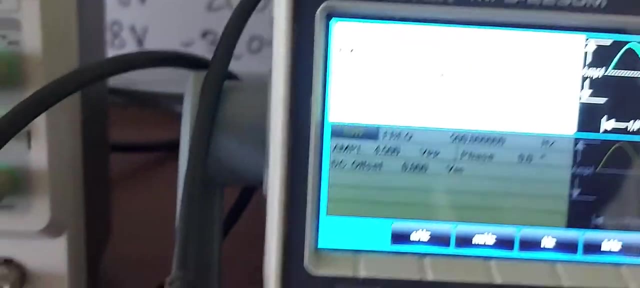 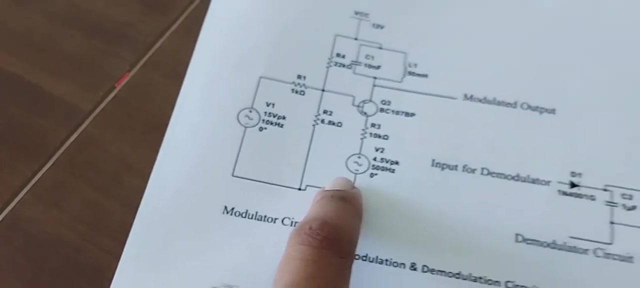 frequency is low and carrier signal low and carrier signal frequency is high. so right now, if you will look at the display, this channel one is of message signal and its frequency is set to the 500 hertz and amplitude is 4.5 volt. as I have already shown you in this circuit, message signal frequency is 500 hertz and 4.5 volt. 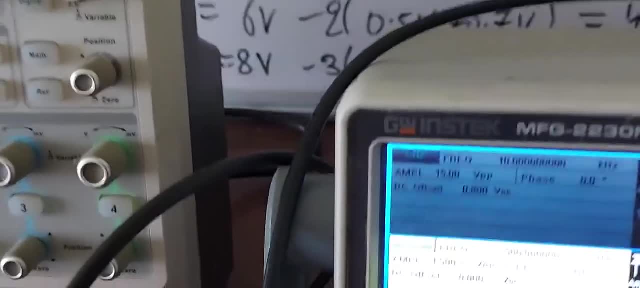 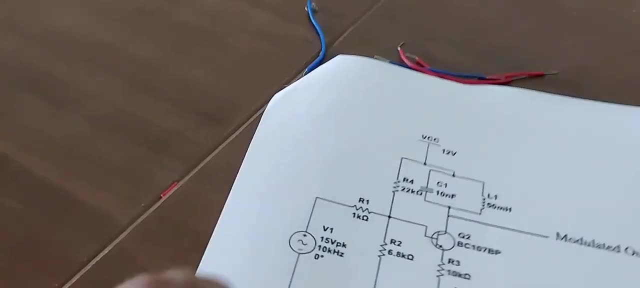 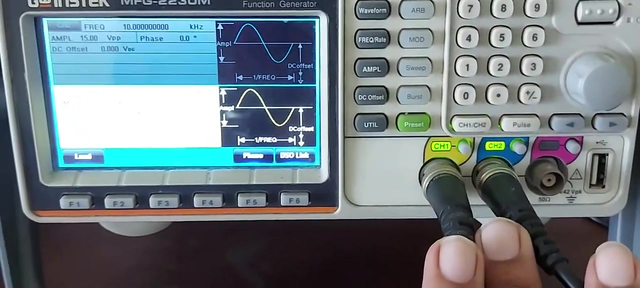 and if we will switch, then you will see here this channel two is set on frequency 10 kilo hertz and amplitude 15 volt. as you can see in this circuit, 10 kilo hertz and 15 volt and this using these two channels, we will give the input of message and carrier. now 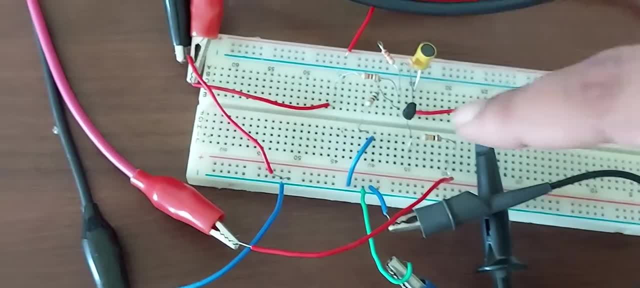 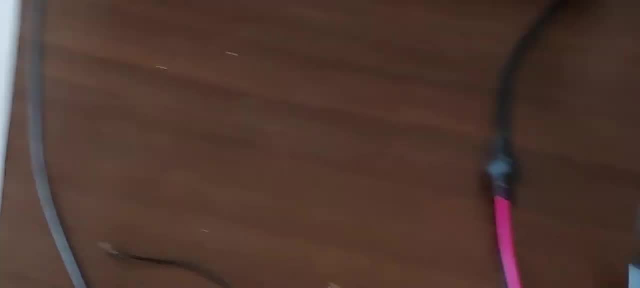 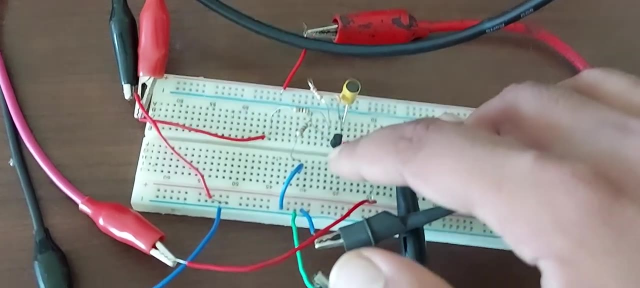 you can see here we have connected this circuit. this black one is our transistor. we do not don't have exactly this transistor, so we are using 2N555 transistor. So it is not perfect transistor for the AM modulation, but this is available with us right now so we are using it. 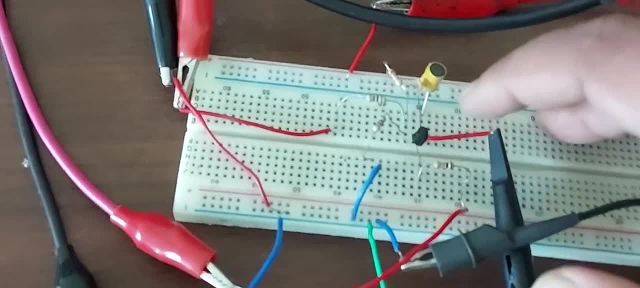 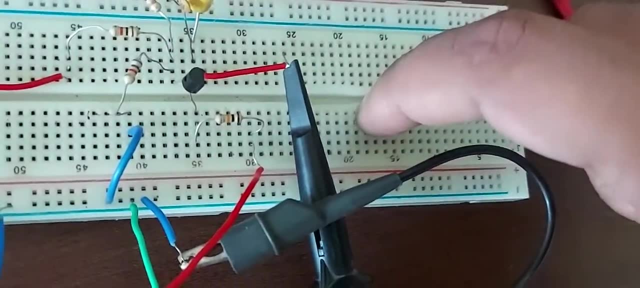 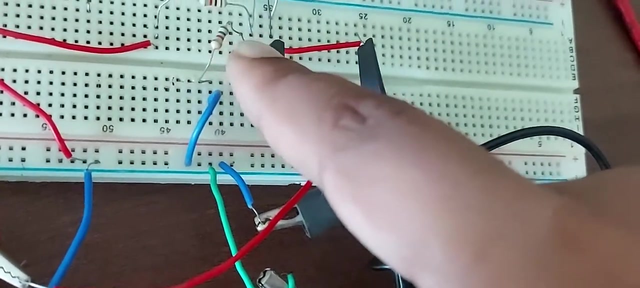 and other than that, this emitter, base and collector has been connected here. this is the breadboard. as you know, this is the breadboard, this side is the collector of this transistor, this middle one, this side is the base and this lower one is the emitter, as you can see from. 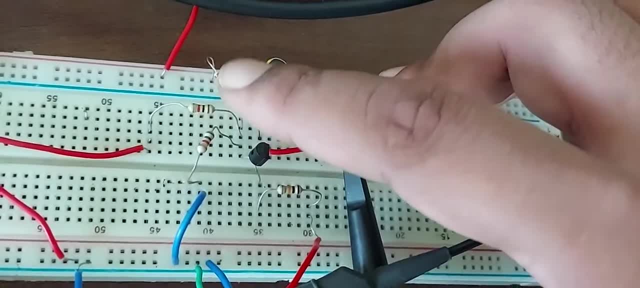 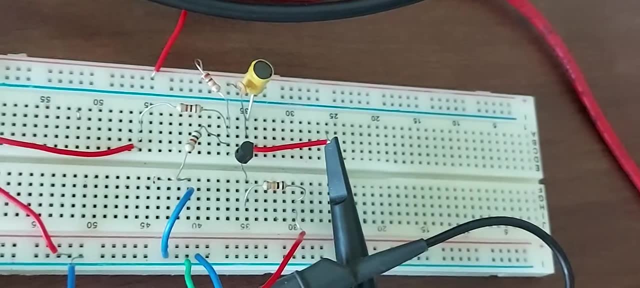 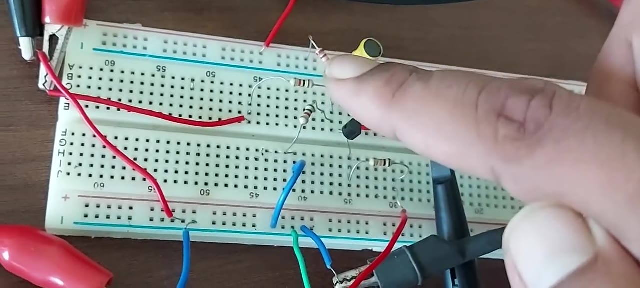 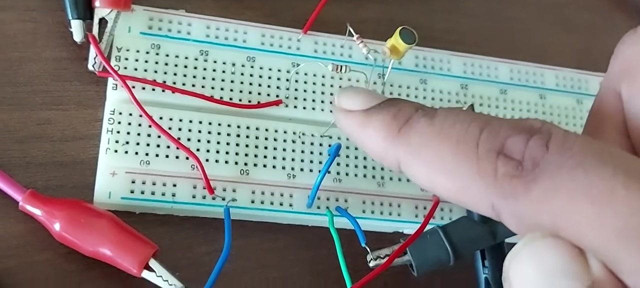 collector. I have connected one. this, this small one. this is small one. this is the capacitor, this is the, this is the inductor- yellow one- And from base I have connected one 22 kilo ohm resistance. This middle one is 1 kilo ohm resistance and this one is 6.8 kilo ohm. 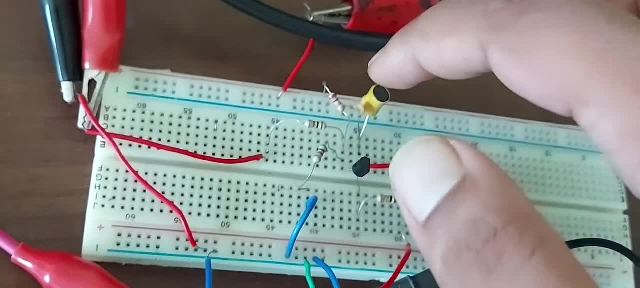 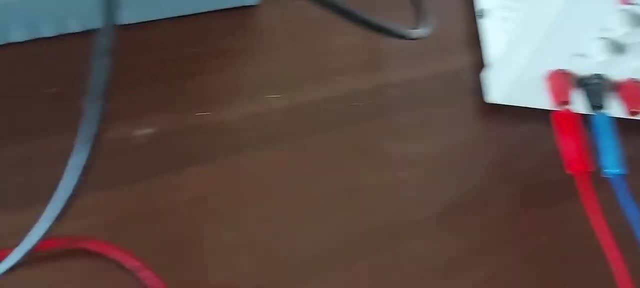 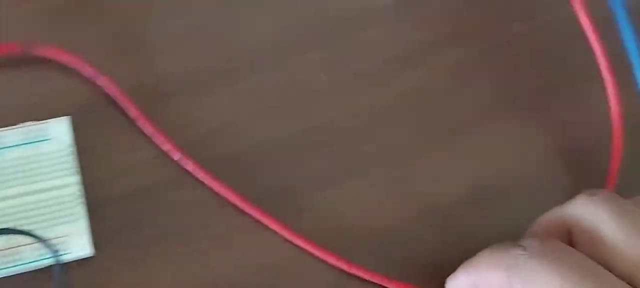 And from here at this point, we have connected one power supply using this DC source. I have switched it off right now because I am explaining the circuit, I am touching the circuit. at this point We have to switch off the DC power supply. So this is the DC power supply plus and this is the DC power supply minus. 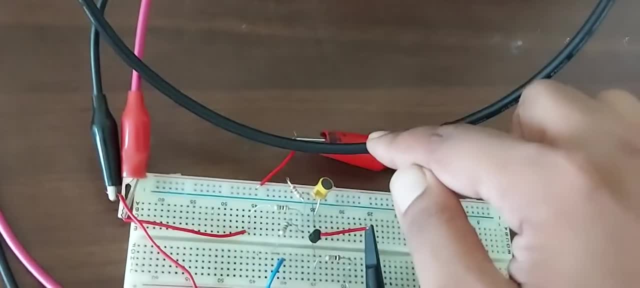 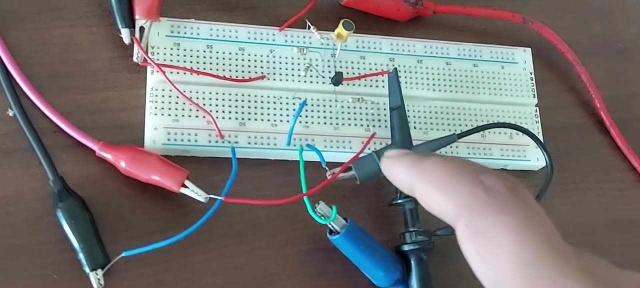 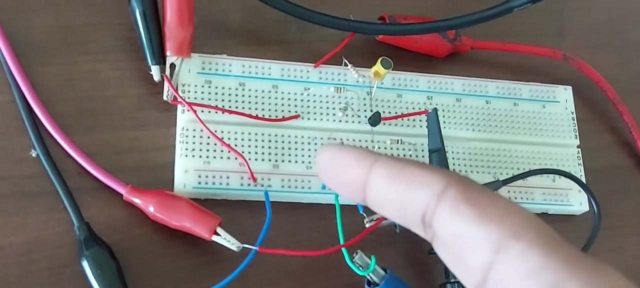 So we have connected minus here and plus here at this. So these lines are already sorted of breadboard and these lines are already sorted of breadboard Horizontally sorted and in this middle one we are vertically sorted. So I have connected this resistance. 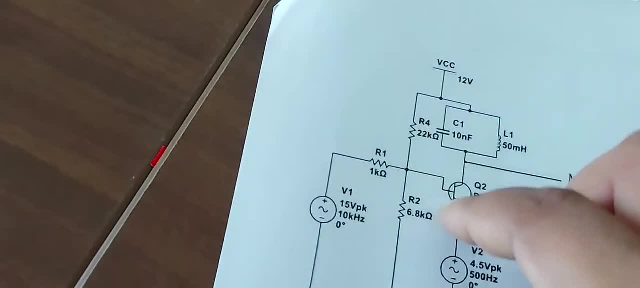 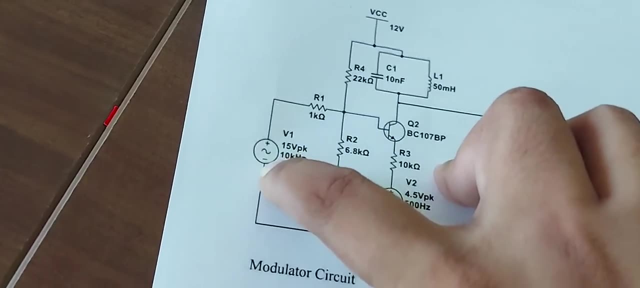 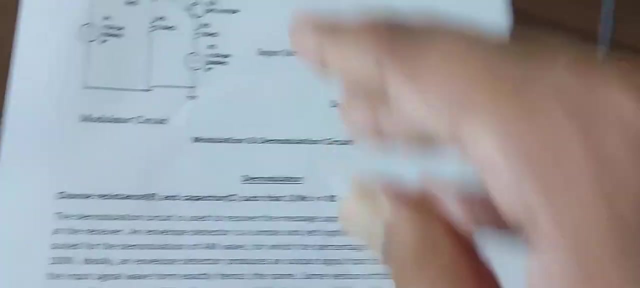 As it is shown in the circuit. you can see this, this, this, all this resistance, as we saw, In which 1 kilo ohm is connected to our carrier signal and this lower 10 kilo ohm from emitter is connected to our message signal. 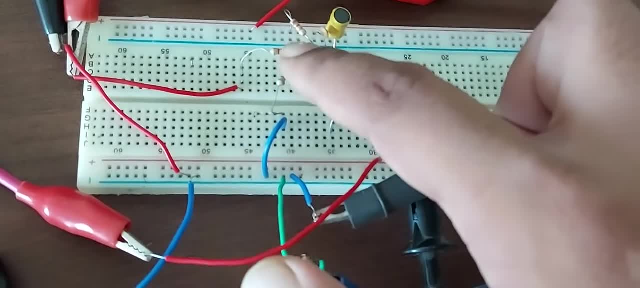 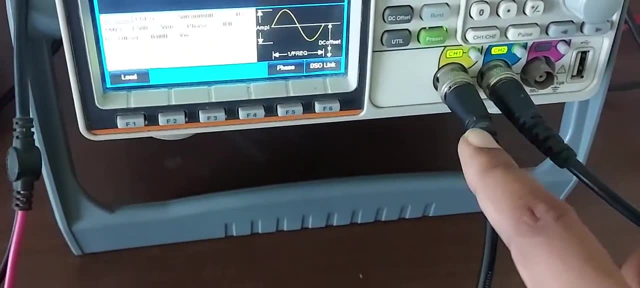 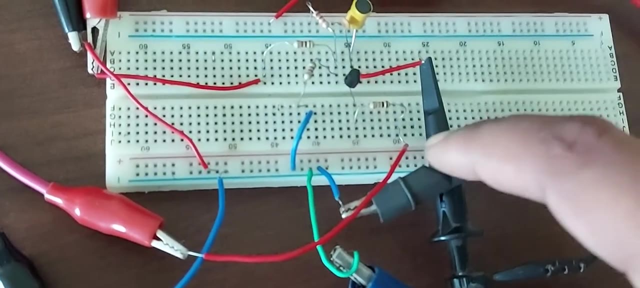 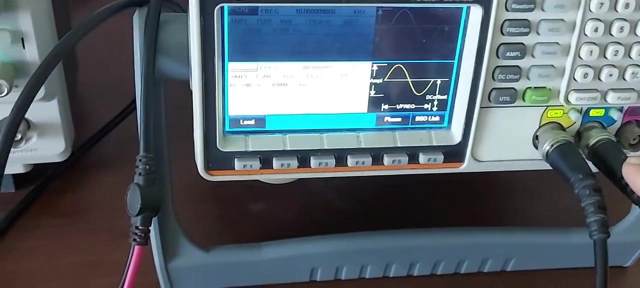 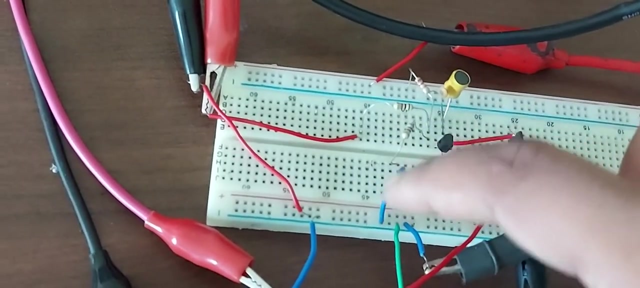 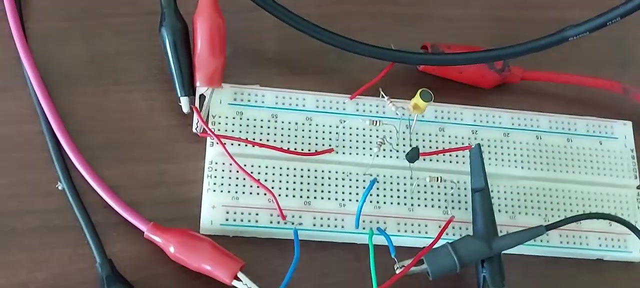 As you can see, this is my 1 kilo ohm, which is connected to the carrier signal channel 1 of the function generator. Okay, and this is the emitter. this is emitter and this is the 10 kilo ohm resistance from which I have connected this channel 1. channel 2, which is of message signal- okay, from function generator, and we have connected this wire to make it to the ground, and this is the plus volt and this is the minus volt and this is how we have connected our circuit. 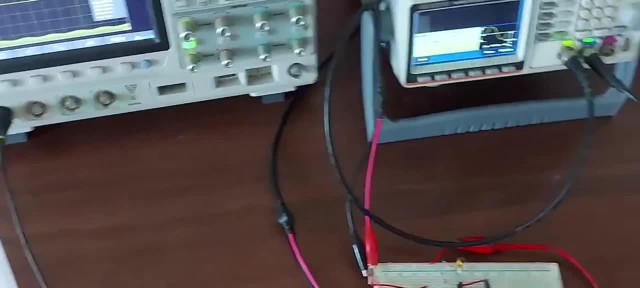 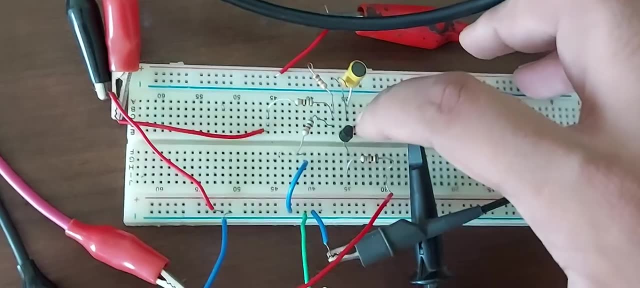 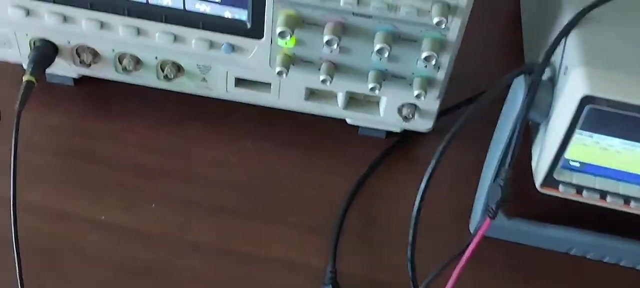 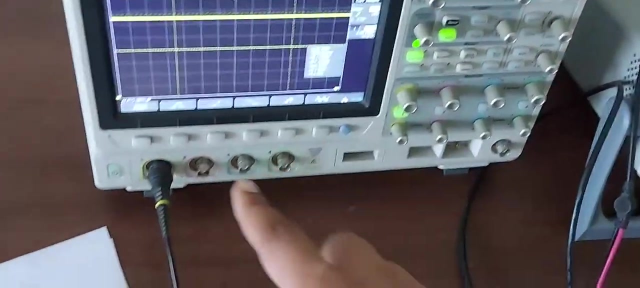 Okay, Now what we will do. our desired output will be the am output. and yeah, one more thing from emitter side, sorry, from collector side, from here, this is the dso. we have connected dso channel. so our third is this dso, where we will observe our waveform. so this dso, this is one channel, this is 4 channel dso. simultaneously we can observe 4 channel dso. 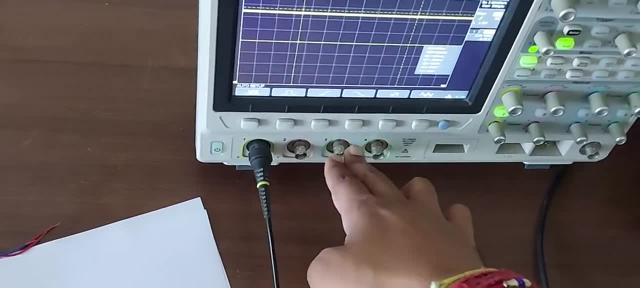 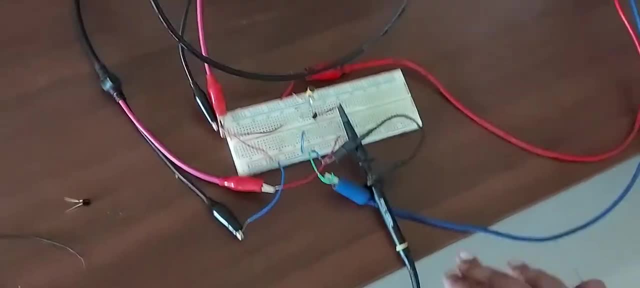 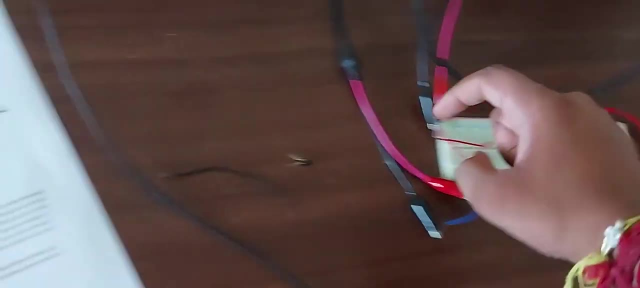 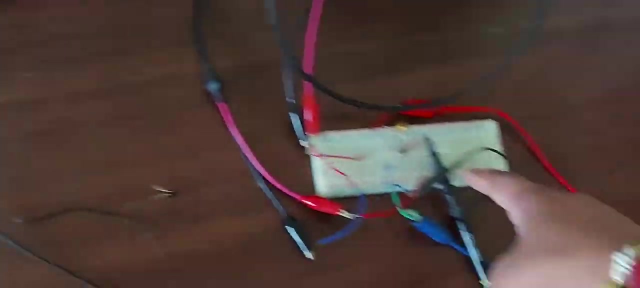 We can observe 4 outputs here from 1, 2, 3, 4. okay, but we don't need 4 channels right now, we need only one. so we have connected this through this cable. we have connected it at the collector side. as you can see this shown in the output at collector side, modulated output is coming out. so there, we have connected the dso and we will observe the output in this dso. 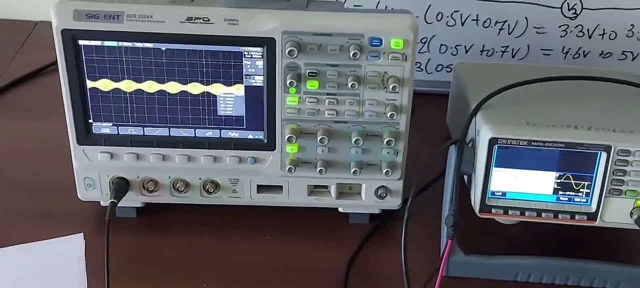 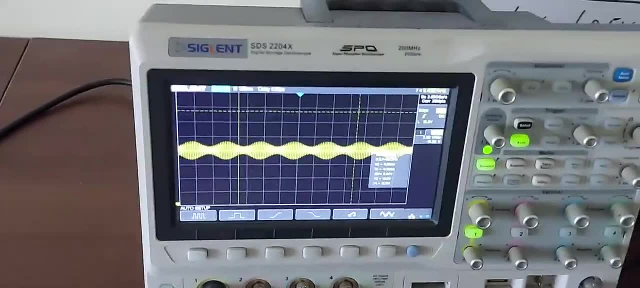 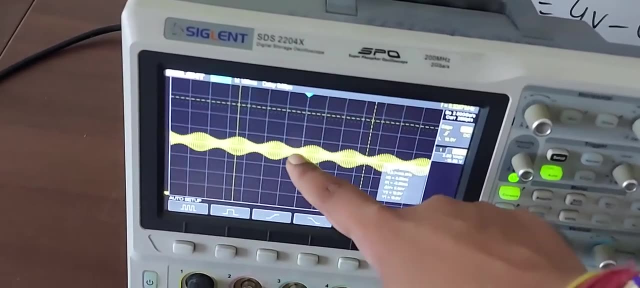 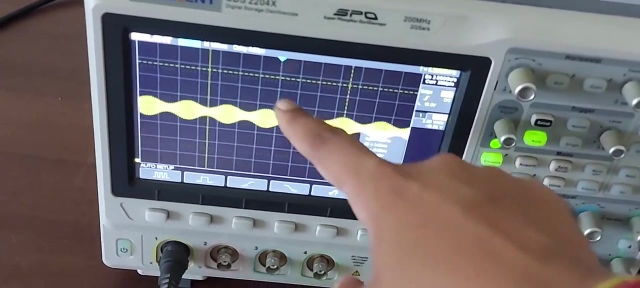 Okay, Okay, so this is the output. we get the modulated output of fm. okay, as you can see on this display, this is sorry- modulated output of am. as you can see, this is the envelope. okay, it is envelope like of upper, upper level and lower level. okay, when we do the demodulation, when we do the demodulation, 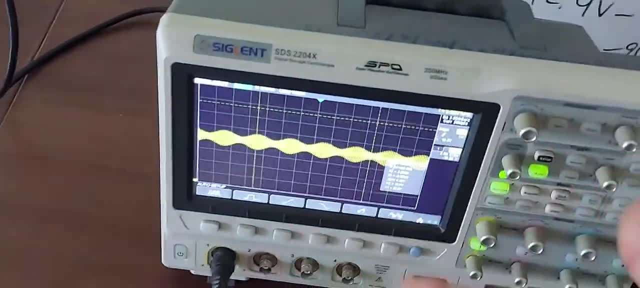 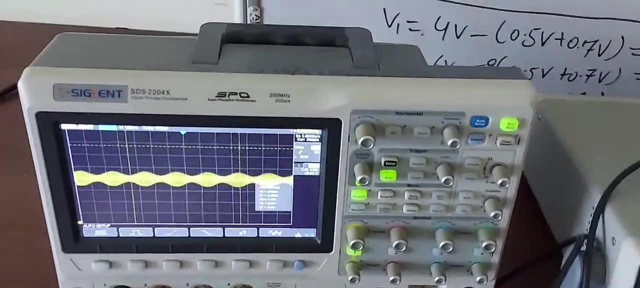 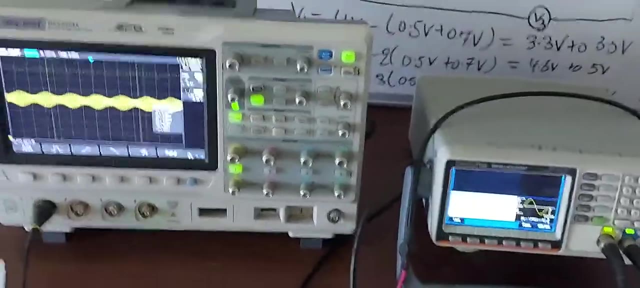 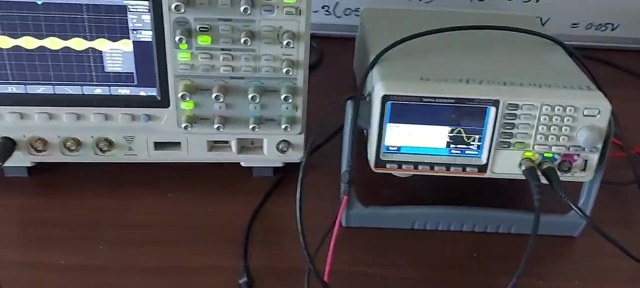 And at that point we detect this envelope. there is one process called envelope detector. using that we do the demodulation. but right now we are doing only modulation part. so you can see here: so this is the am modulation setup and this is our output. and now if we want to change the modulation index, then what we will do- modulation, how we can change the modulation index. 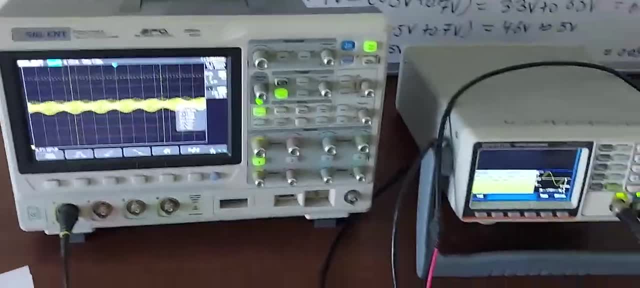 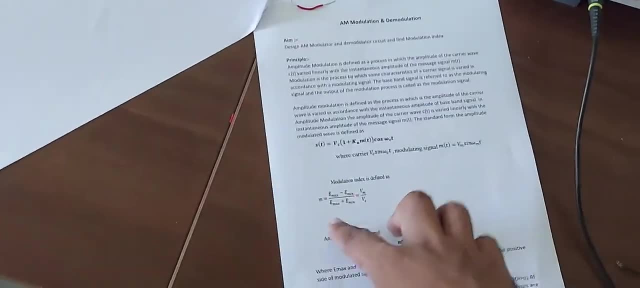 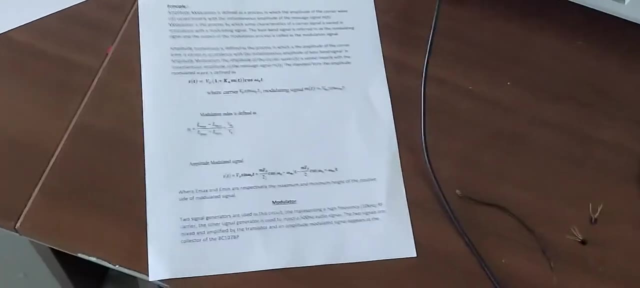 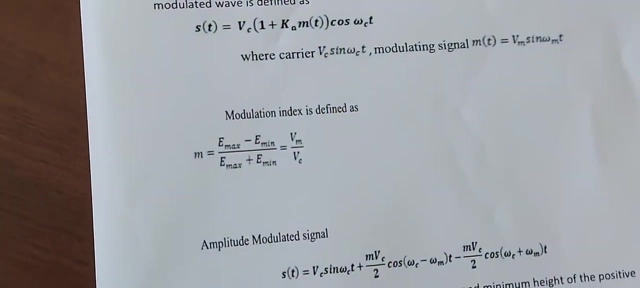 Okay, Okay. Okay. So this is the modulated индex where emax minus emin by emax plus emin. you can see here- this is our modulation index formula. what is emax? here you can see from this graph, this is the maximum value. 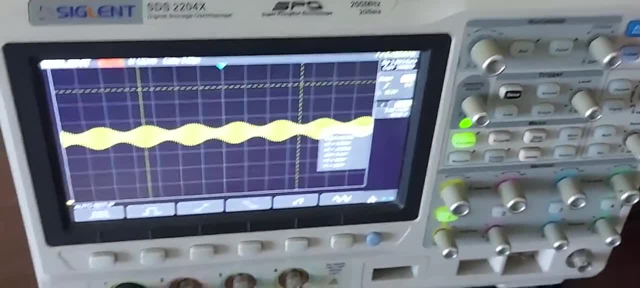 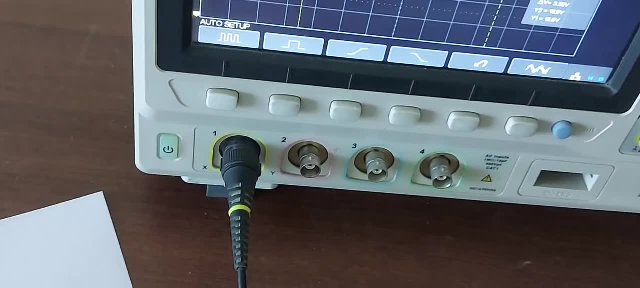 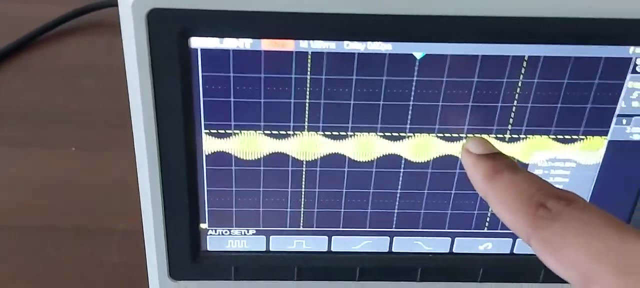 I will first stop this At one point. Okay, So you can see the maximum value. I will bring the cursor down. Okay, See This. This, This is our maximum. This, This is our maximum And wait, Maximum. 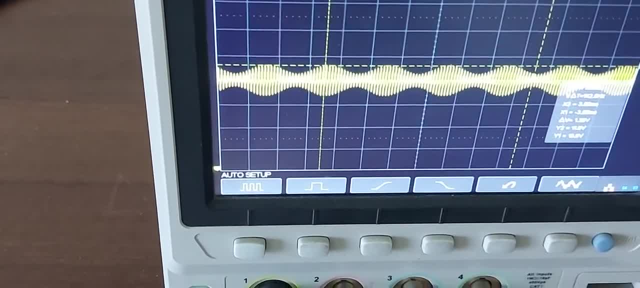 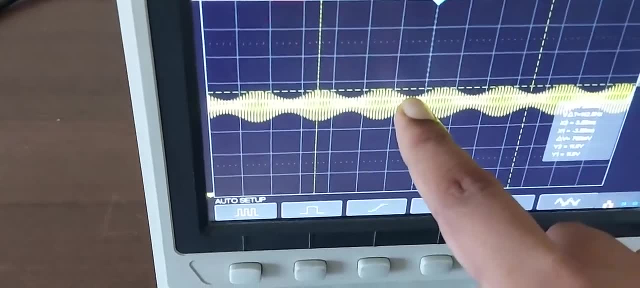 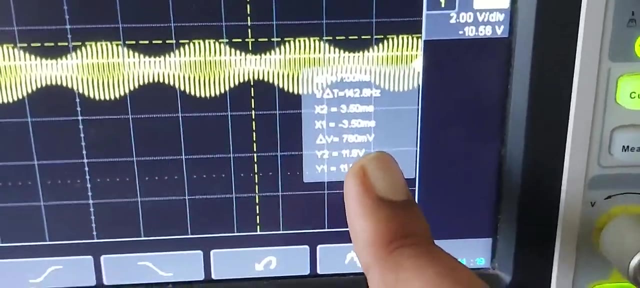 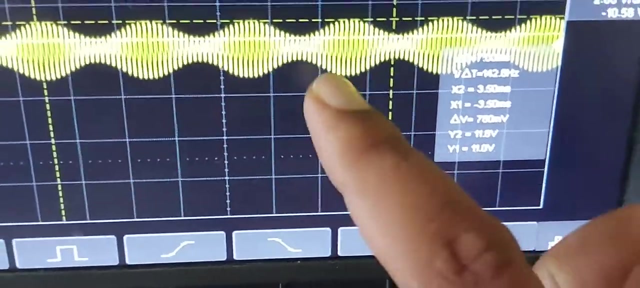 And this is our minimum. This, This lower, lower one. This is our minimum. So I can measure this using cursor and you can see the output here. This Y2 is on 11.8 volt. Y1 is 11 volt, Means this lower part is on 11 volt. This upper part is on 11.8 volt. 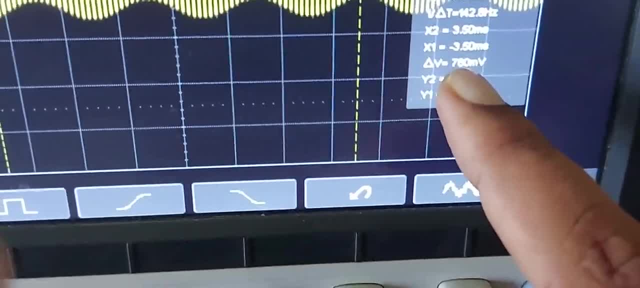 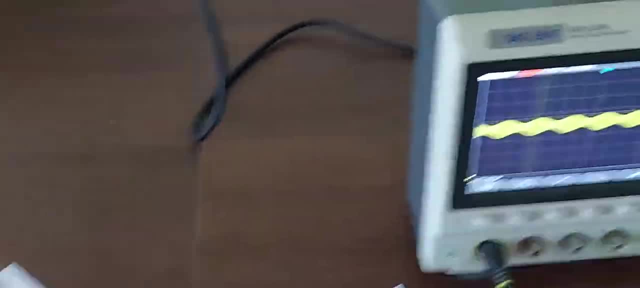 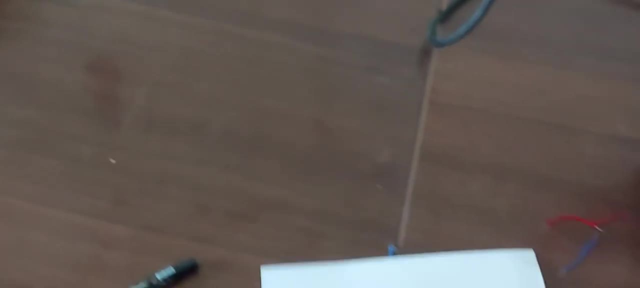 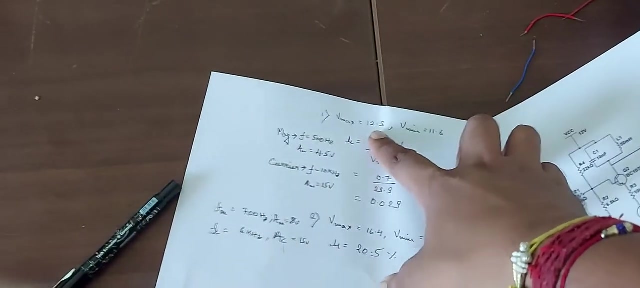 And the difference is 760 millivolt Means about 2.8 volt. It is about 0.8 volt, You can say, And so if we will imply the formula here, Then we will get very low modulation index. I have calculated something In which I got first Vmax 12.3.. Right now I am getting Vmax 11.8.. 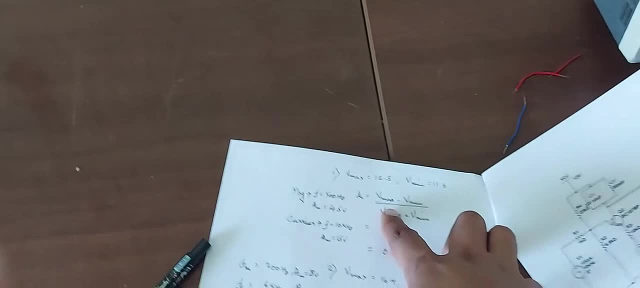 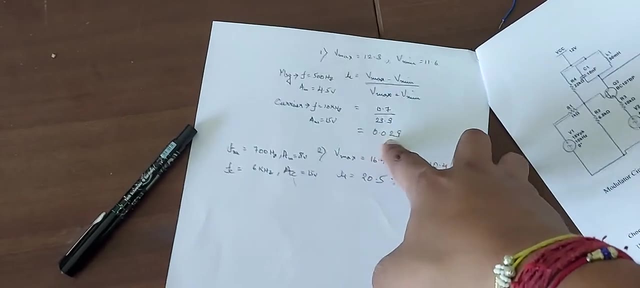 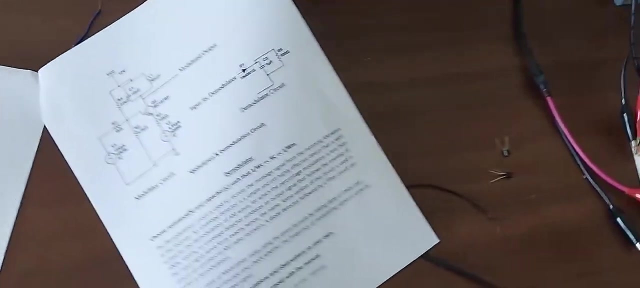 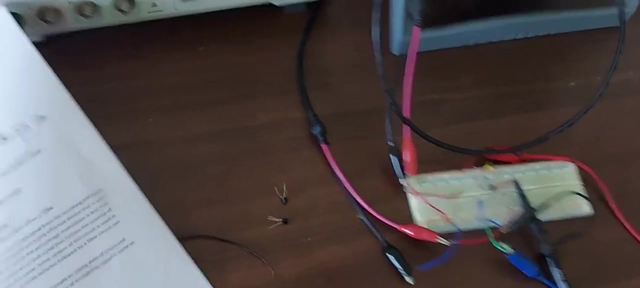 But It doesn't matter, It's okay, No problem with that. So, using this formula, If I will calculate the mu, Okay, Then it came at 0.029.. Means about 2%, Which is very low, Because we are not using the designated transistor. We don't have right now that transistor, That's why we are not using that. But if we will use the 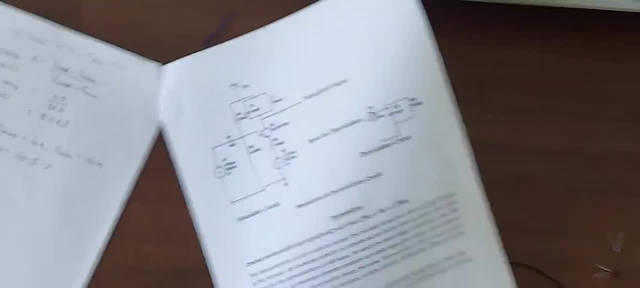 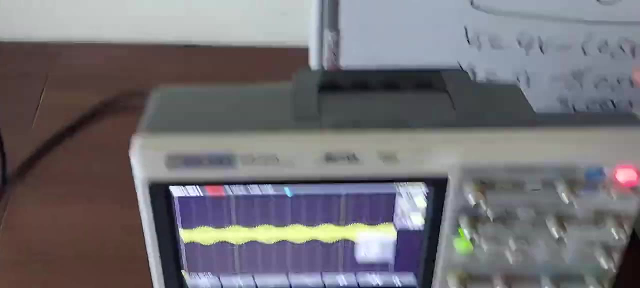 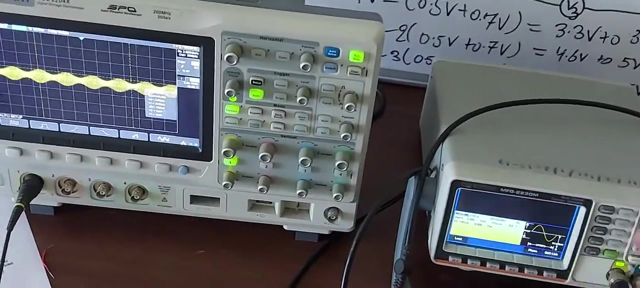 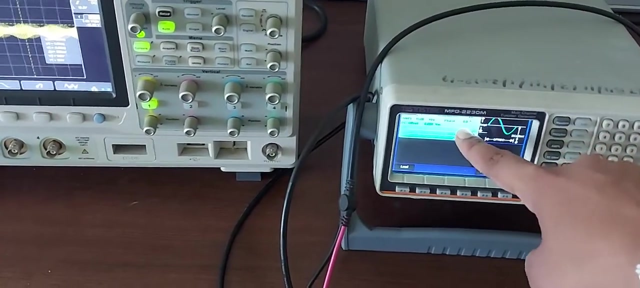 Same transistor as it is given here. Okay, Then we will get the desired output. So, right now, What we can do, We will change this modulation index. You can see here in this graph When I I will change this frequency of carrier. Okay, Okay, I will change this frequency of carrier Of channel 1.. Then 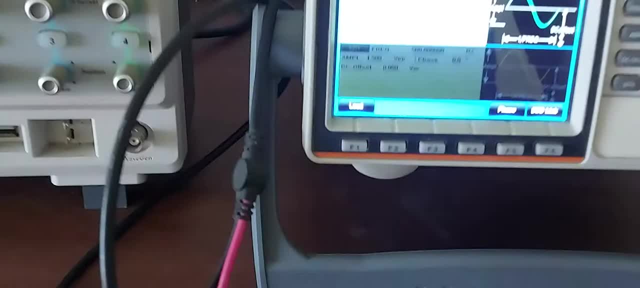 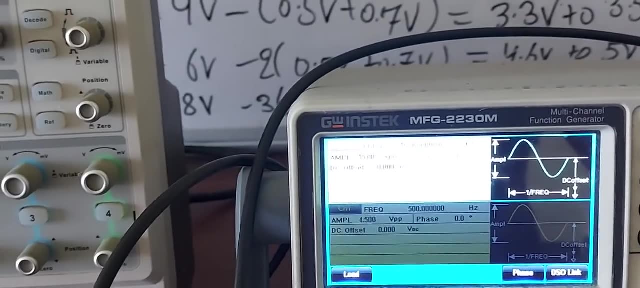 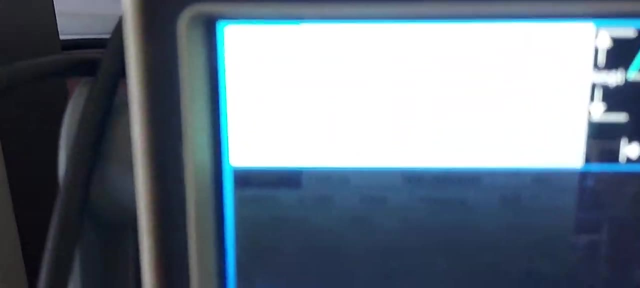 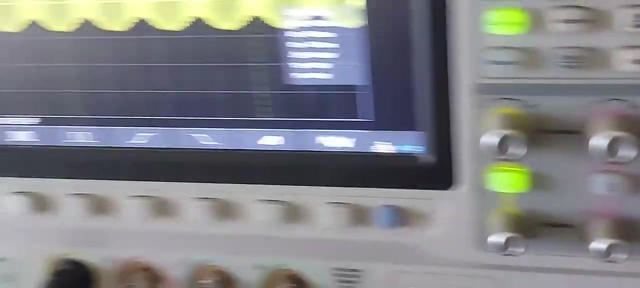 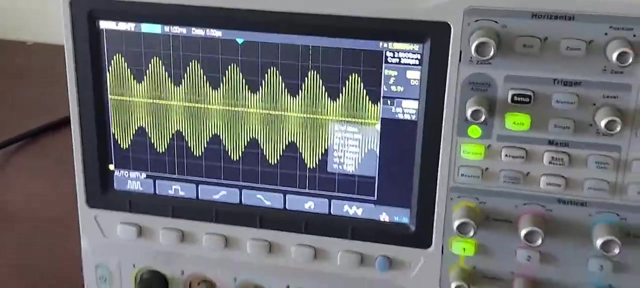 We will get. Right now, it is on 10 volt. I am going to change it. I am going to reduce it. Okay, I am going to reduce it. See, it is on 10 volt, I am reducing it. I make 9 volt right now And you see the changes. I am reducing it. You can see the changes. Okay, My output change. 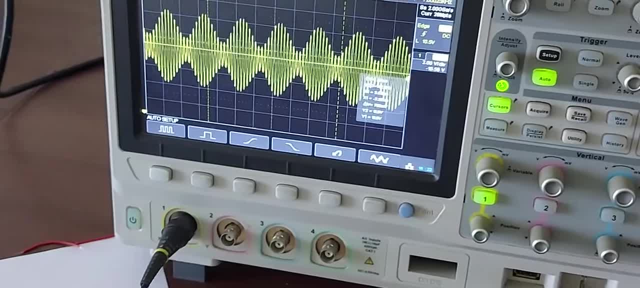 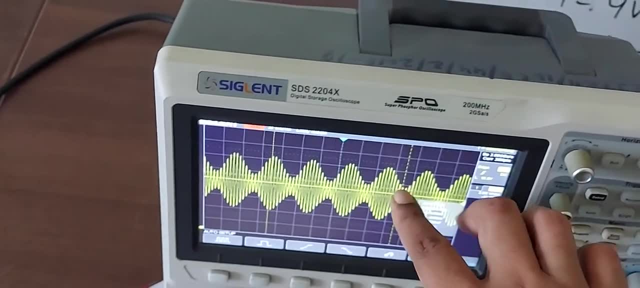 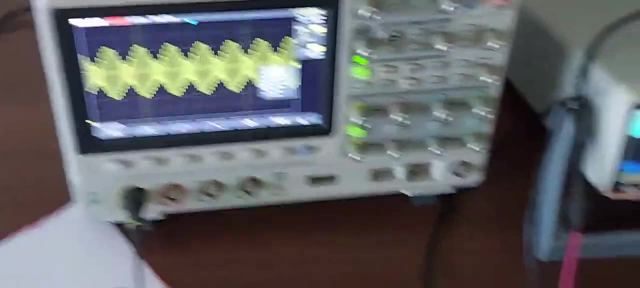 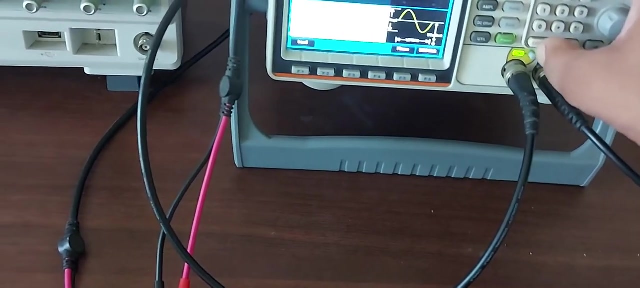 Modulated output changed. Okay, So my modulation index also changed Because this gap, Because this gap In between this gap, This changes, So modulation index changes. So this is how. Or we can do one more thing: We can change the message signal frequency also. From there also we can observe the changes. 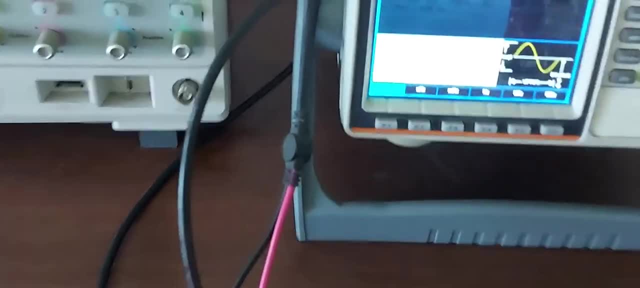 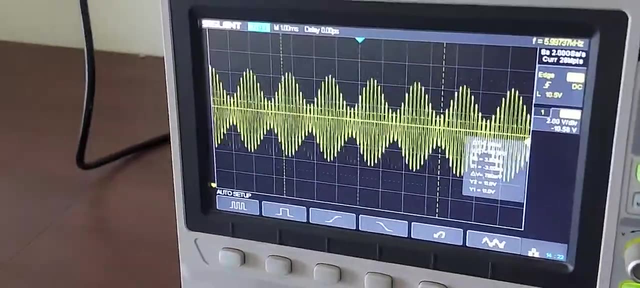 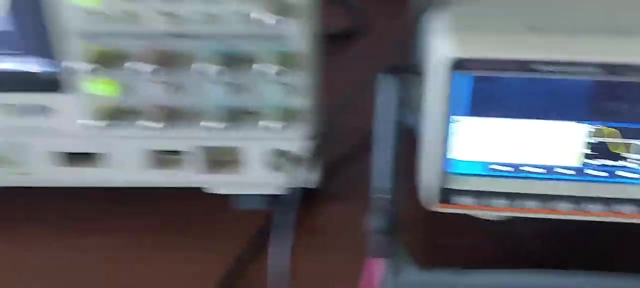 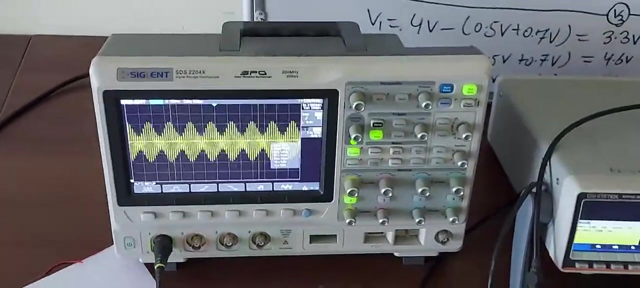 If we will change the message signal frequency- It is on 500 hertz right now- If we will increase this And you will see these changes. There is little bit changes, But there is changes. Okay, Even changing the amplitude also, We can change this output of AM modulator. So this is how we achieve desired modulation. 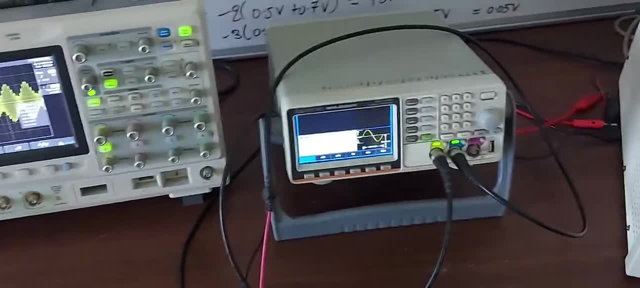 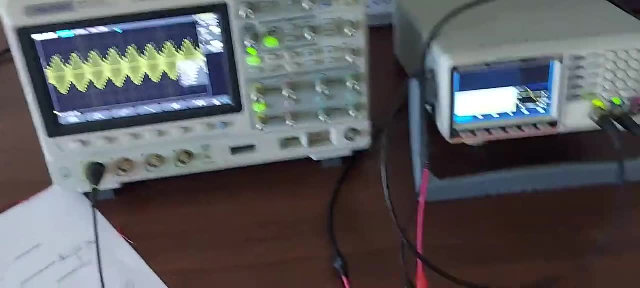 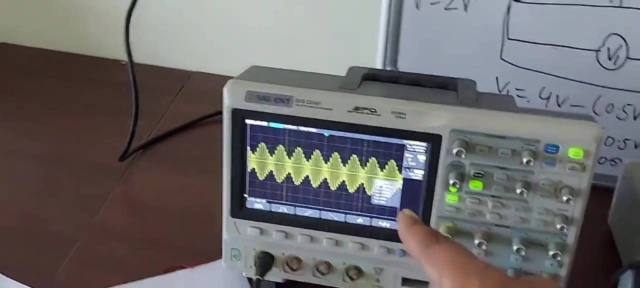 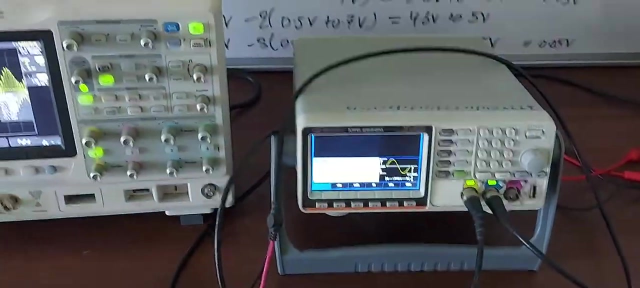 Modulation index. You have learned in your theory classes What is modulation index and why it is needed. So this is how we implement AM modulation And this is how we see the modulated signal In our DSO. Okay, This is function generator. This is DC power supply. That's it for today, Thank you. 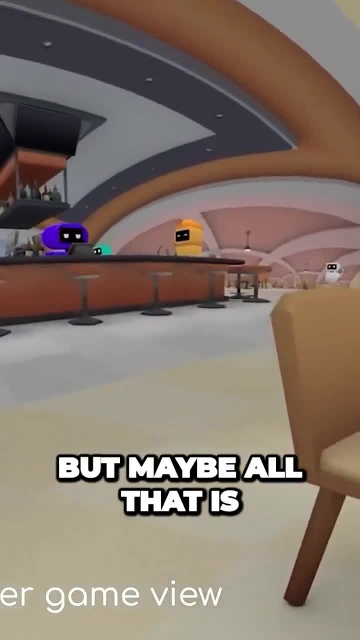 Scientists try to explain that with dark energy, but maybe all that is happening is that the universe is just naturally hyperbolic in its shape. So what would that mean if the universe really was hyperbolic? It would mean that the universe was really infinite, The flat space we. 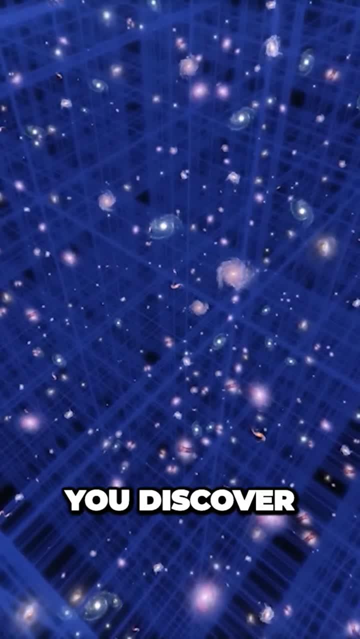 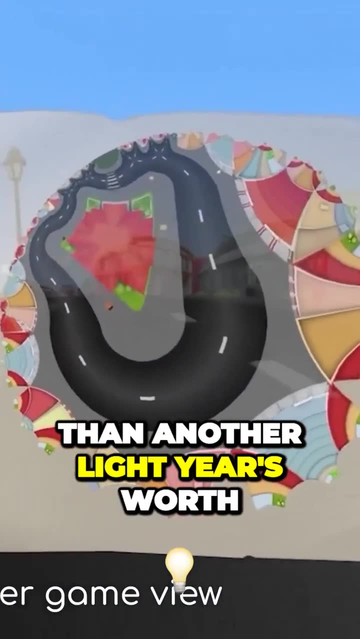 looked at was infinite. For each light year you travelled out, you'd discover another light year's worth of space. However, with hyperbolic space, you'd discover more than another light year's worth of space. It's like opening infinite doors, except inside each door are two new ones.